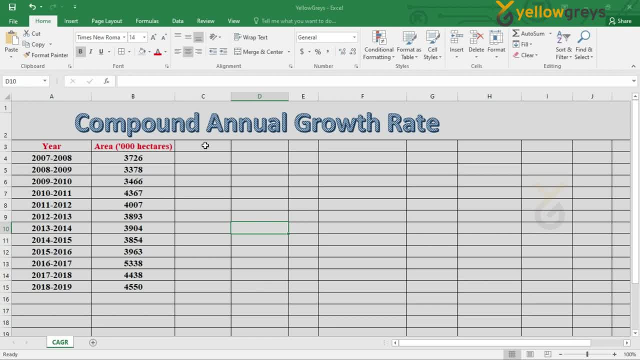 Before estimation we have to differentiate the data into dependent variable and independent variable. In this example, the independent variable x is time, Which is nothing but 1,, 2,, 3,, 4,, 5,, 6, up to 12.. 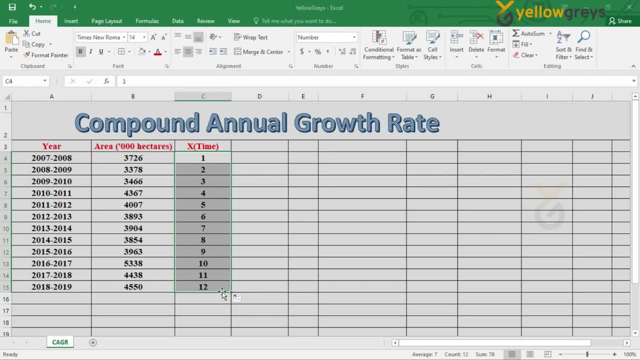 Which represents the number of years from 1 to 12.. Dependent variable y represents the log value of the particular data which we had taken. Because the estimation of compound annual growth rate is based on exponential function, To estimate log we have to type equal to Ln. 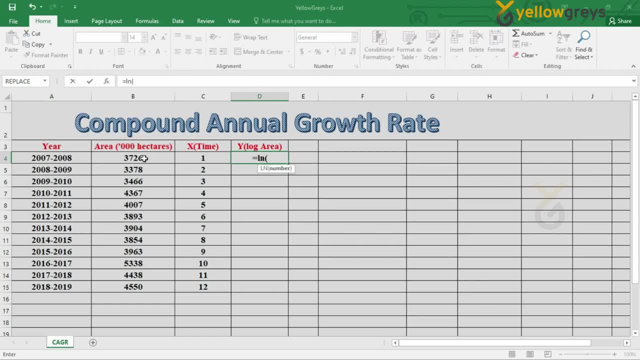 Open the bracket. Select the cell reference of the text in which the data is present. Close the bracket and press enter. Drag the cell. in order to get the log value of the remaining data For the obtained dependent and independent variable, we have to run regression. 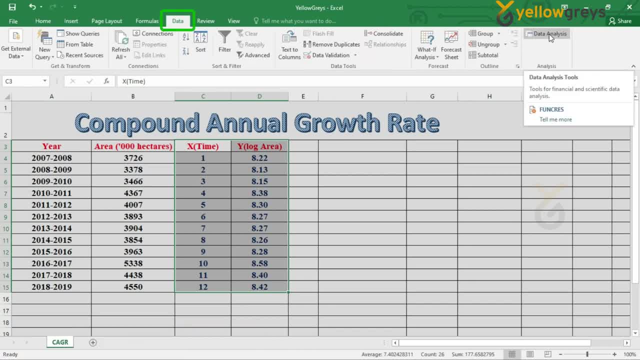 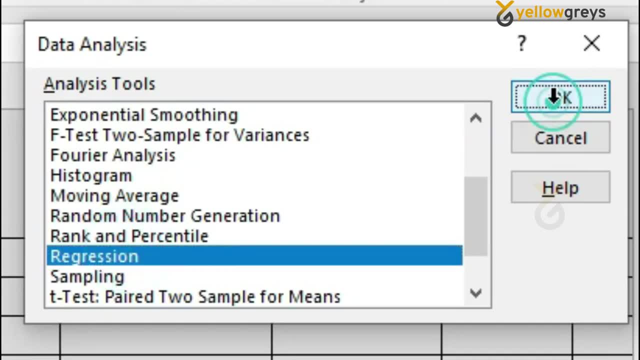 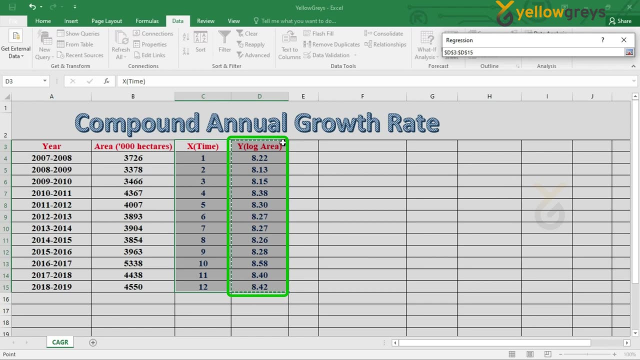 For that. select data in the data analysis From the analysis tools we have to select regression, Then click ok. In input y range we have to select the data of dependent variable. That is log area. In input x range we have to select the independent variable. 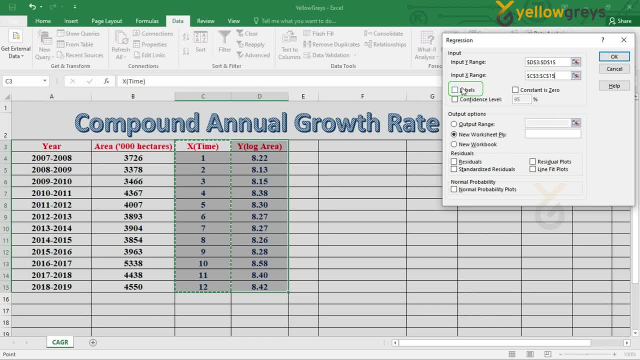 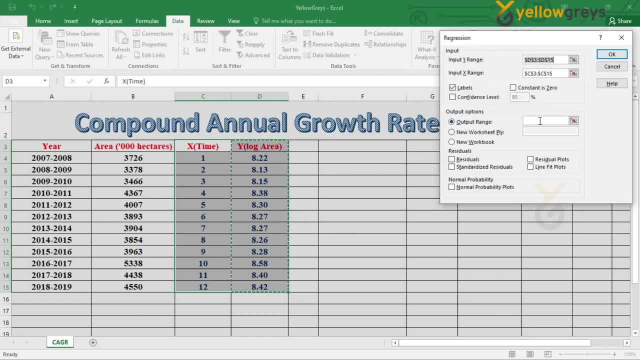 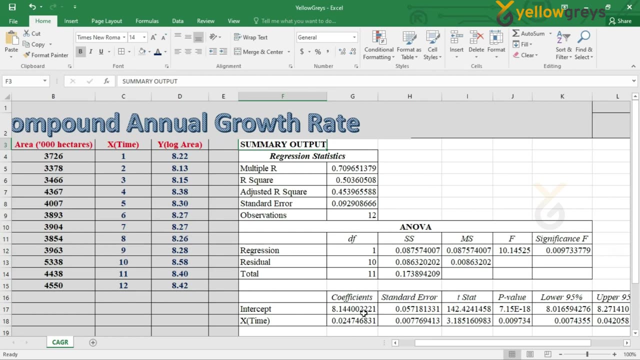 That is time. Then select labels, as we have selected the values, including the labels. Then select the output range where you have to place the result. Then press ok. Here we will get the results of regression statistics, ANOVA and different coefficients. 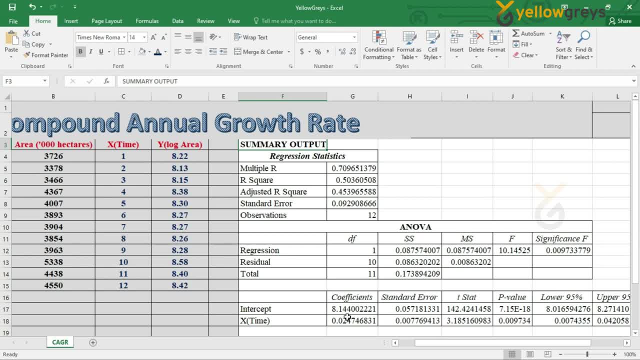 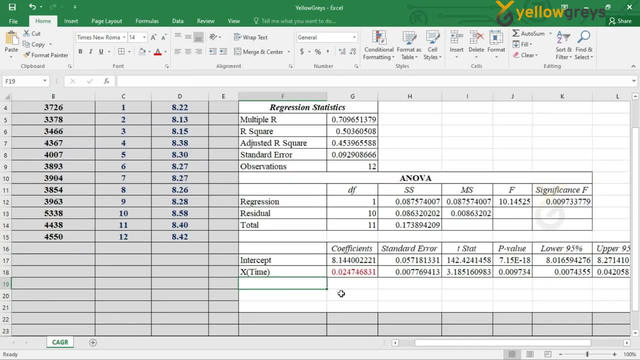 In order to estimate CAGR, we need the coefficient of time variable. This is the coefficient of time variable. To estimate CAGR, we have to find out the antilog value for the independent variable coefficient by using the function exp, That is, exponential function. 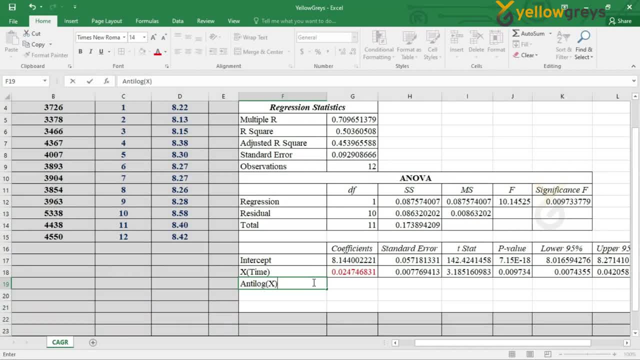 Antilog of independent variable Equal to exp. Open the bracket, Select the cell reference, Close the bracket and press enter. To find out CAGR, we have to subtract 1 from the antilog value, and which should be multiplied by 100.. 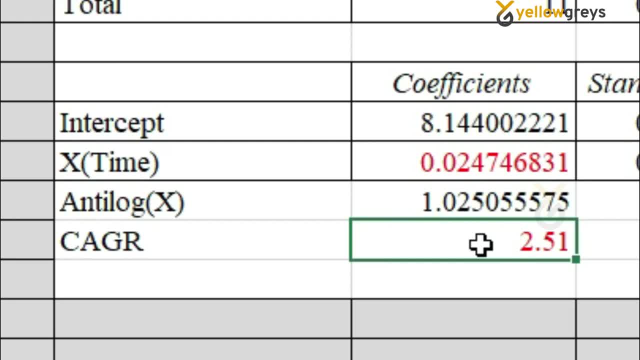 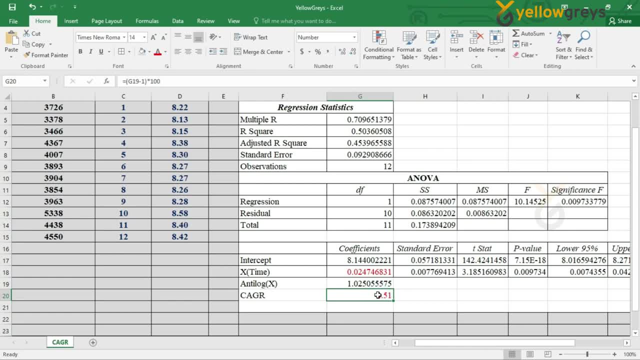 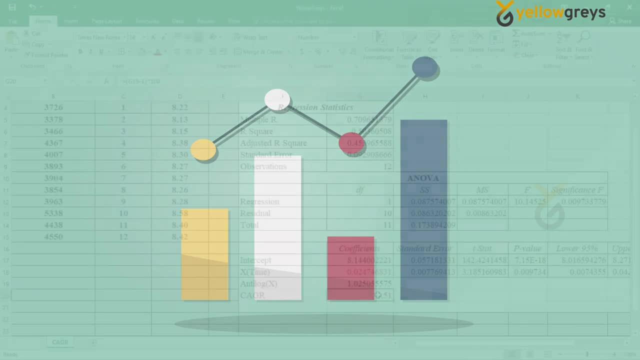 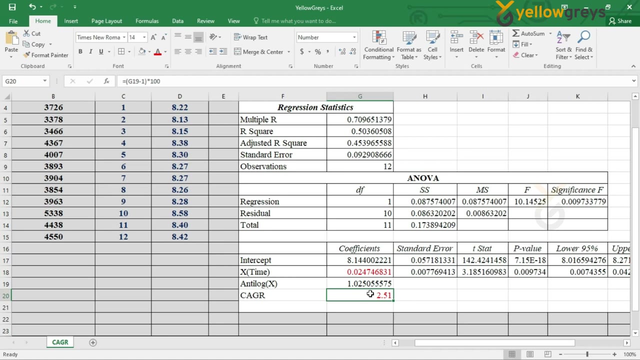 The value which we obtained represents the value of CAGR. It is interpreted as: over the period, the area under PGNP in India is increased at the rate of 2.51%. And also one more thing we have to represent whether the CAGR is significant or not. 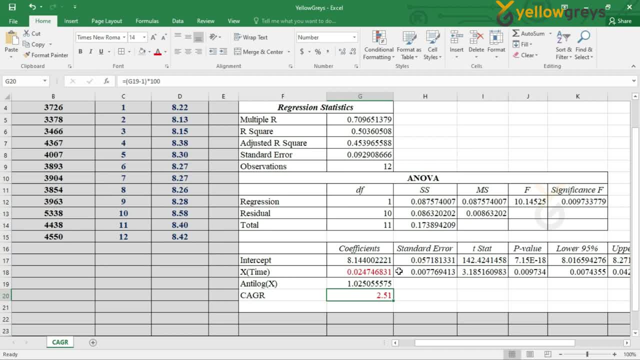 at different level of significance. In order to check the level of significance, we will use the value of P. If the P value is less than 0.05, then it is significant by 100.. If the P value is less than 0.05,. 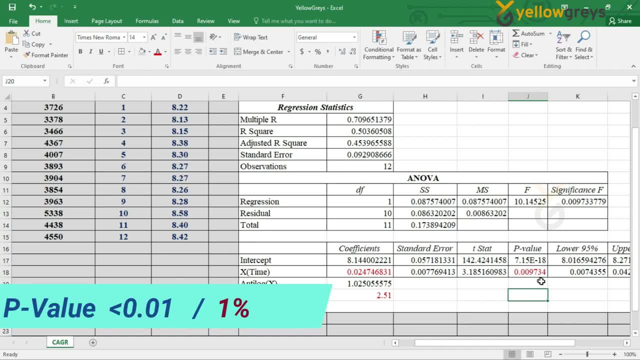 then it is significant by 5% level. If it is less than by 0.01,, then it is significant by 1%. In this example, the obtained value is significant at both 1% and 5% level. Here. 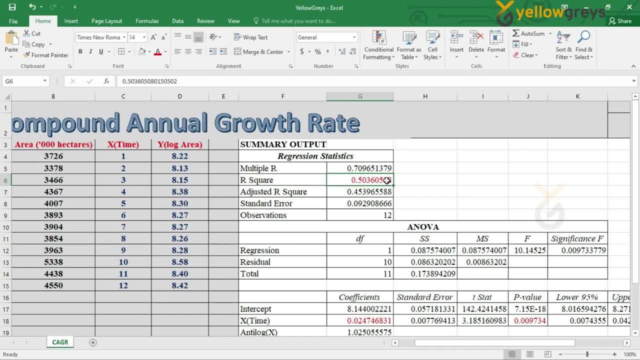 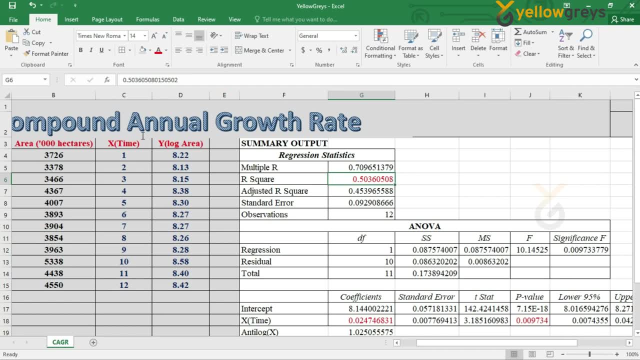 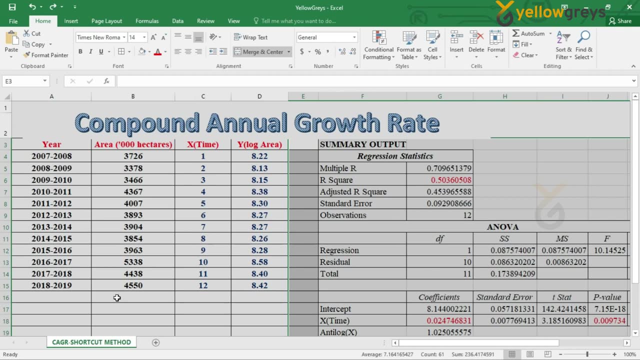 the R-square value was 0.50, which indicates that 50% of the variation in the area was was explained over the years. Now I will show you the shortcut method to estimate only the CAGR value. After getting the value, let's cross check with the regression method and the shortcut method. 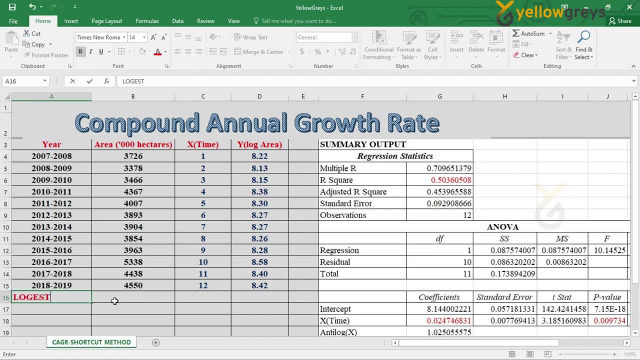 For that we have to find logist value of the selected data that is equal to logist. open the bracket, select the range of the data, close the bracket and press enter. Then find out the CAGR value by subtracting 1 from the logist value and multiplied by 100.. Let's cross check. 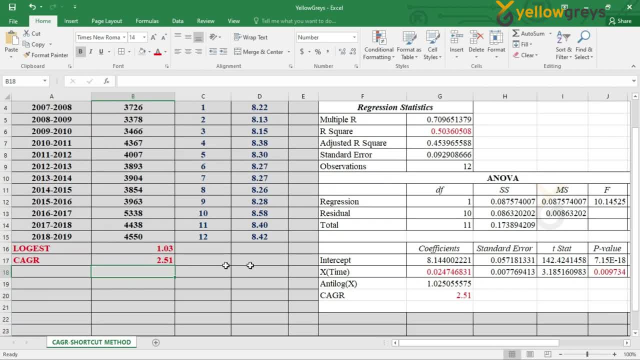 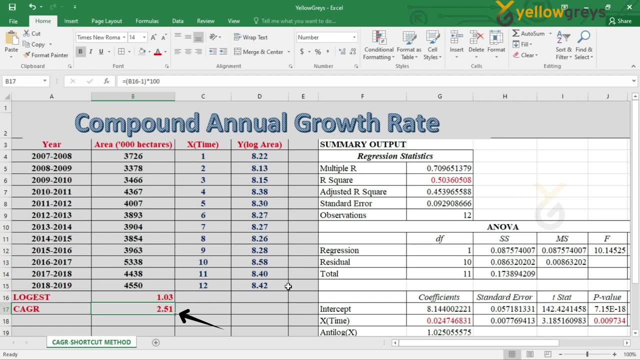 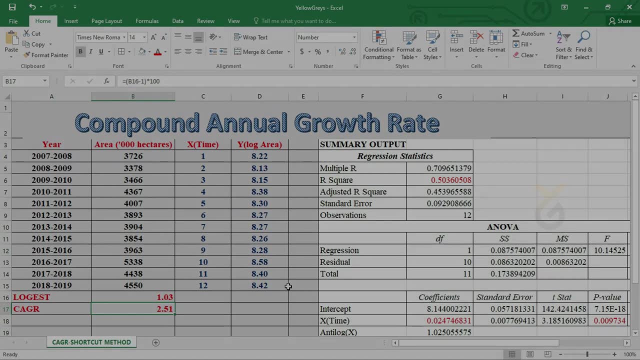 with the regression method and the shortcut method- See, the value of CAGR is similar. I hope now you have understand how to calculate CAGR. Stay tuned for more analysis. Thank you.